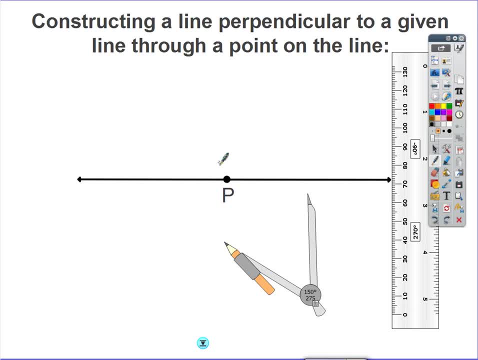 line that's going to pass through point P and perpendicular to the given line. So let's go ahead and take our compass here first, and we're going to put the point of the compass on point P and we're going to draw a arc that's going to intersect the line at two points. So I can stretch. 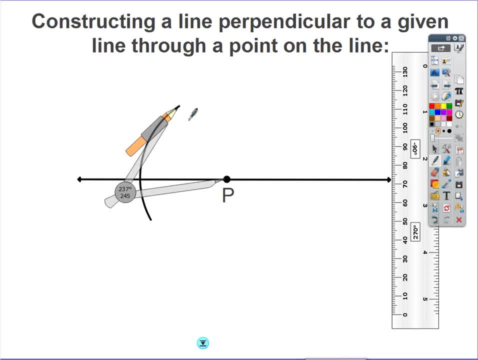 or shrink my compass to whatever I need, and I'm going to draw an arc that intersects the line twice. So when you draw that arc, it should be something that is larger than a semicircle a little bit, so you can see where the intersections are. So here I have. 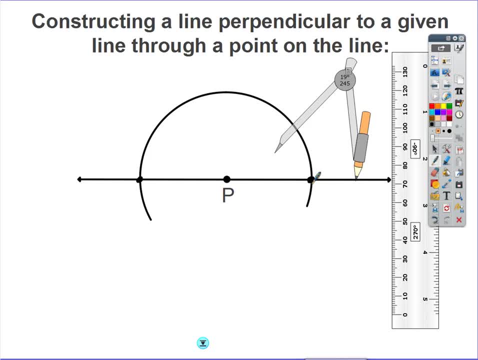 at least a semicircle, and I've created two intersections that are both equal distance from point P. Now we're going to take our compass length that we've already preset right here, and we're going to take it and we're going to stretch it a little bit longer, We're going to make it a little. 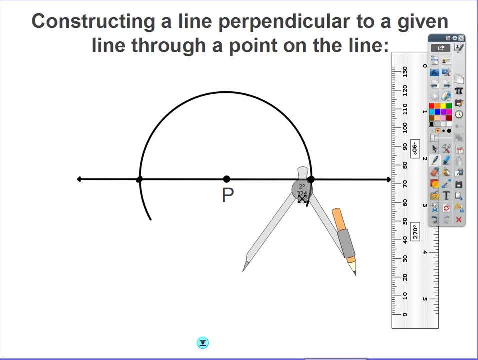 bit bigger than was already given. So here I've stretched my compass a little bit more than it was already. We're going to place the compass point where the arc crossed the line on one side and make a small arc above the line. So here we go. I'm going to go ahead and take my point and let's go ahead and draw an. 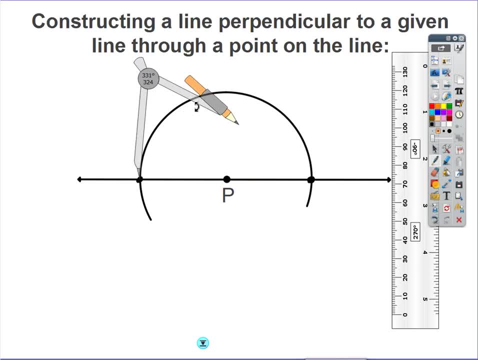 arc. that's a little bit bigger and I'm going to draw an arc above the line here, So I'm going to sketch it an arc there, Without changing the span. I'm going to go ahead and place the compass point where the arc crossed the line on the other side, and when I rotate through here I create another. 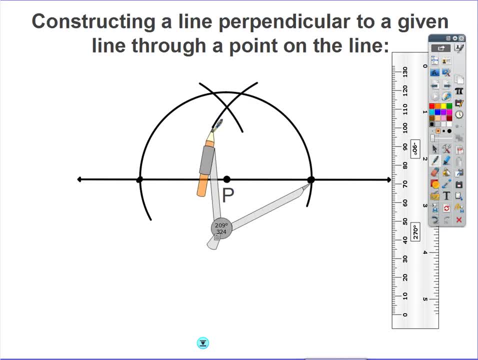 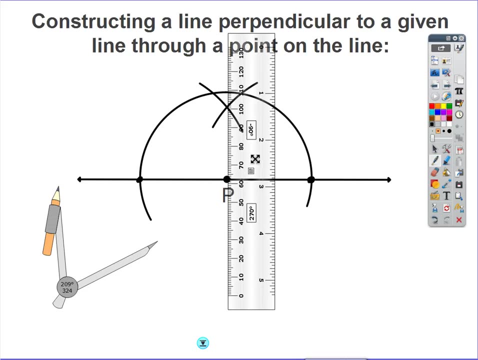 arc, and those two arcs should intersect With your straightedge. now we should be able to draw a segment going through Point P that also crosses the intersection of those two smaller arcs, And this line will be perpendicular to the given line, but it passes through point P. 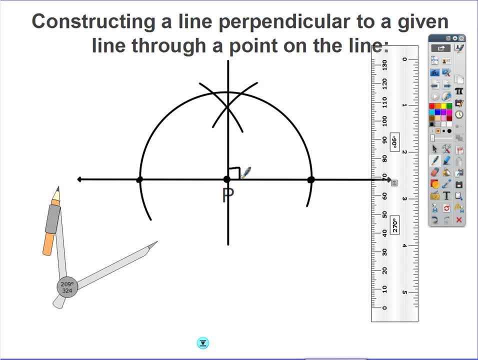 So again, if you want to revisit this video, please rewind to the beginning, watch the steps as we go through it and then try the example problems on your own.